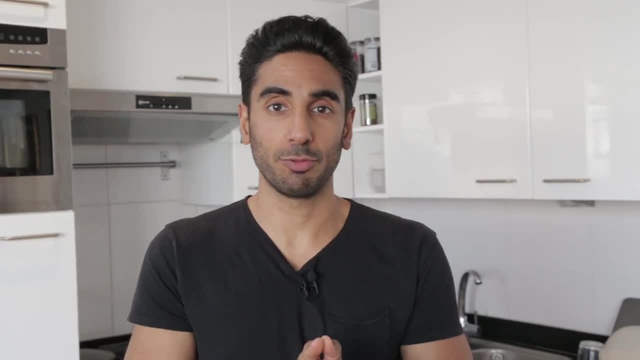 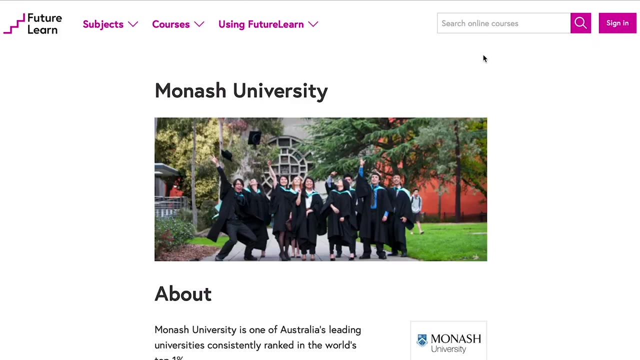 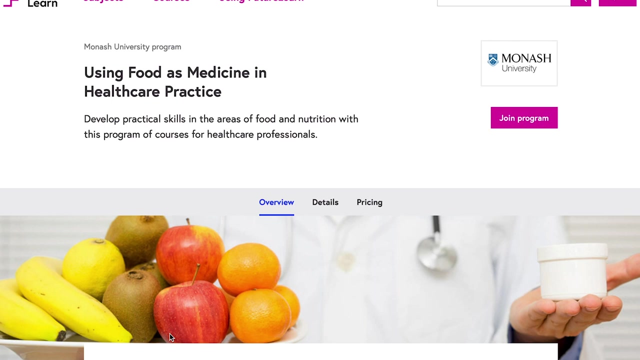 there are a few free courses online that I do recommend. The first is the Food as Medicine course by Monash University, an Australian university. You can get it on FutureLearn and it is free. If you wanted to pay- I think it's around 60 pounds- you'll get a certificate with. 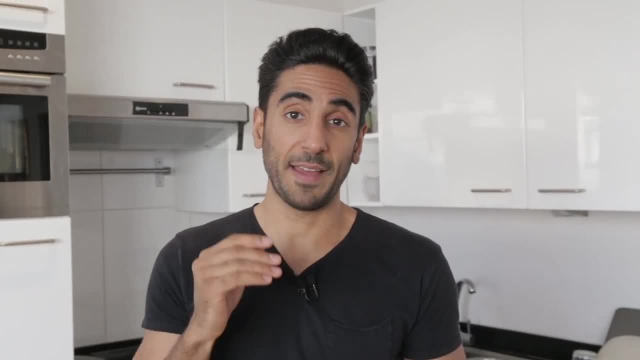 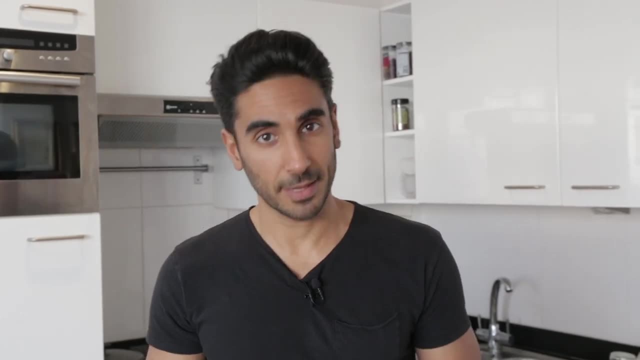 it. but you can do the free course. if you're just dipping your toe and they've got real registered dieticians and doctors talking about the subject and whether food can be referred to as medicine, It can. spoiler alert. The second course I would say is Coursera. So if you look through Coursera, 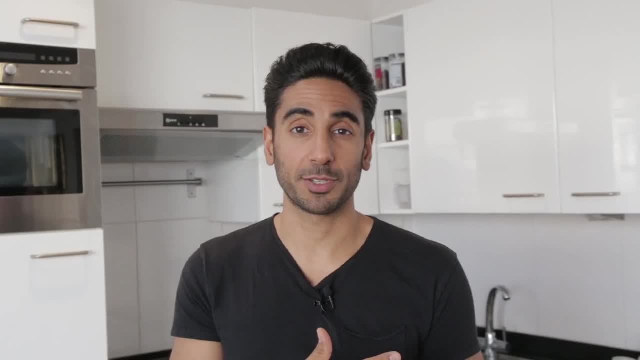 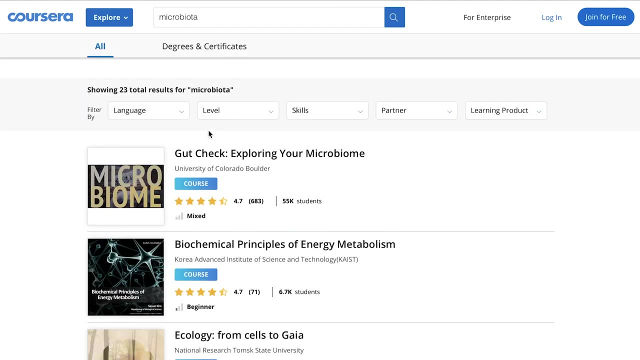 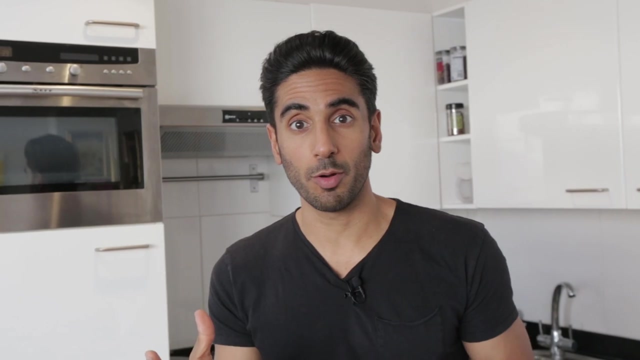 one is by the Knight Lab in West Coast America. They've got a whole course about the microbiota- the population of microbes that live in our gut, and it is absolutely inseparable from health. If you want a more technical dive into the microbiota and how little we know about this, 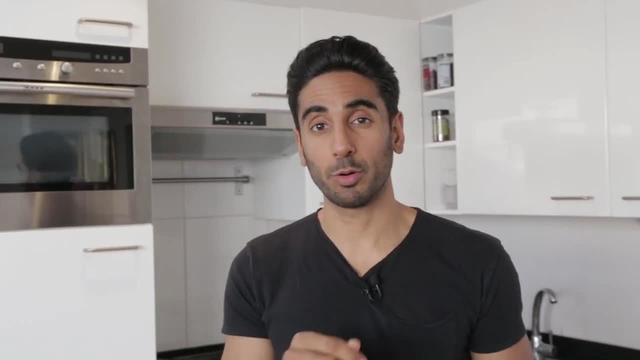 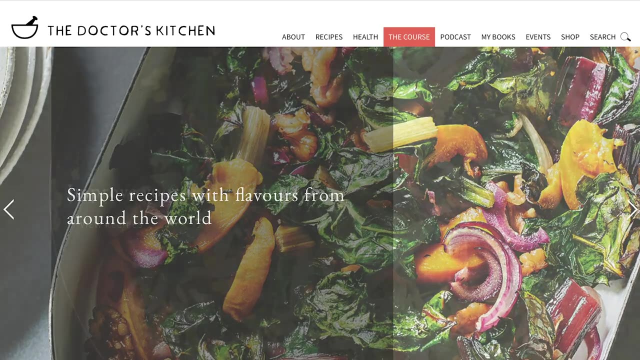 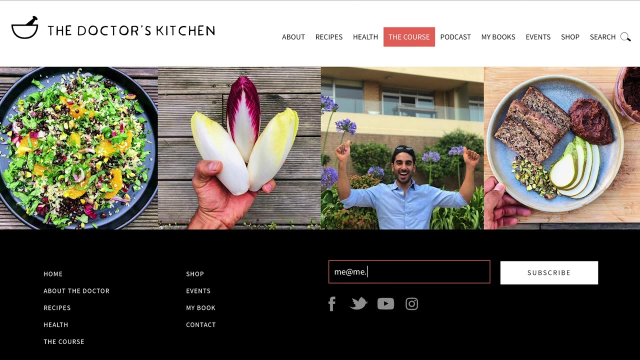 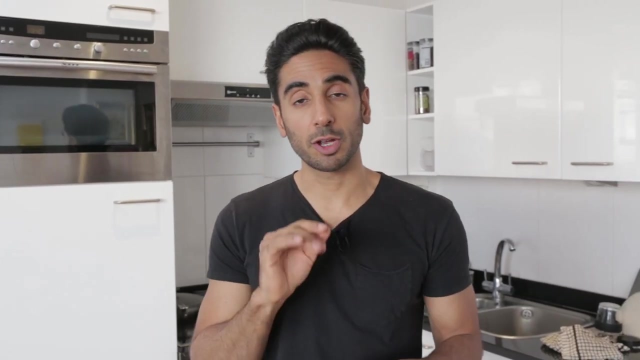 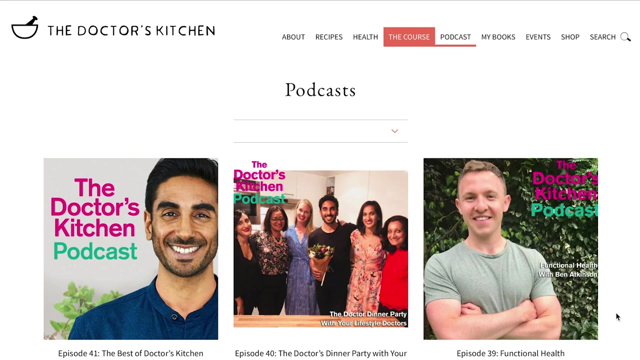 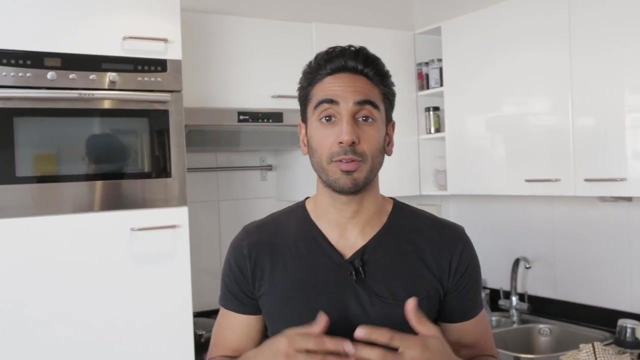 current subject, but how exciting it is. I definitely recommend that course. The links of all will be down below as well. For a basic overview of nutrition, I've got my own course online. You can check that out. I am often asked if there are paid for courses online that people can use to familiarize themselves. 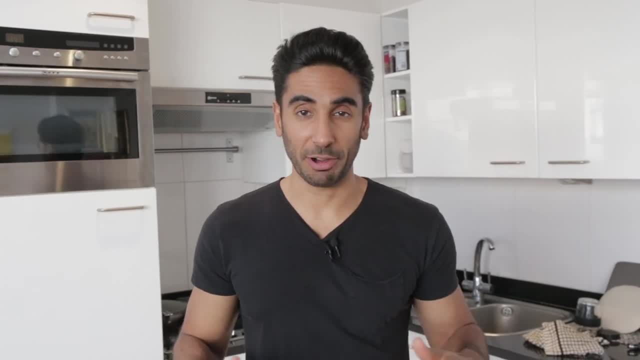 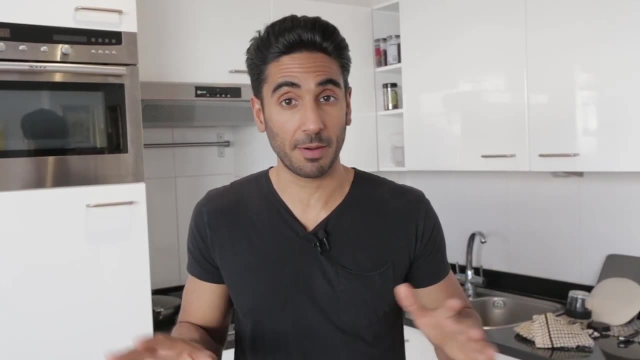 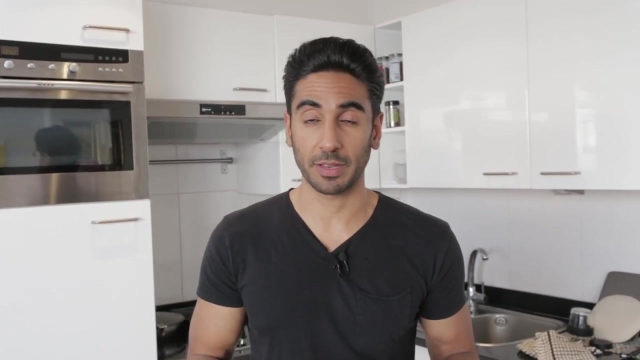 with nutrition in the UK. Categorically, I am not aware of a good course for professionals that is purely online. There might be some, but I'm not aware of ones that I've come across that are worthy of the amount of money that some of these cost, And they range from anywhere between £500 to £2,000. 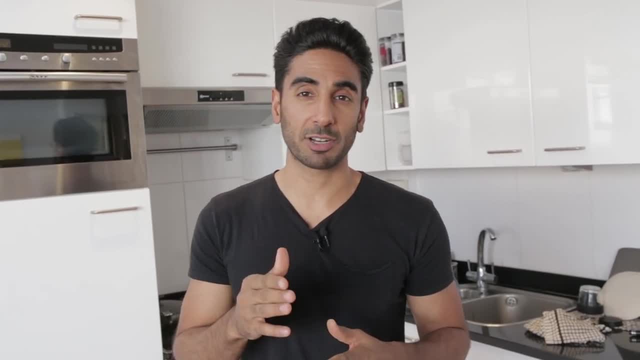 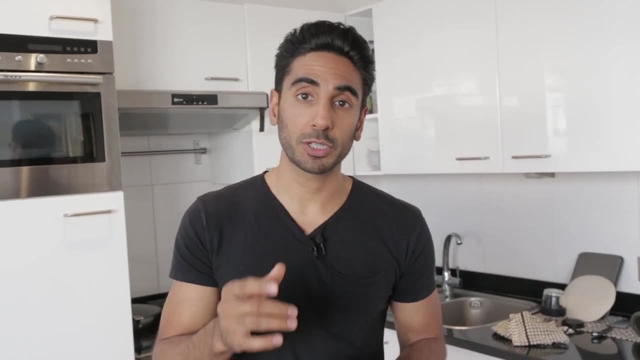 And I just don't think they're worth that amount of money. if you're serious about getting into nutrition research and actually being able to deliver actionable advice to patients, There are courses that I've come across that are worth the money, but I don't think they're. 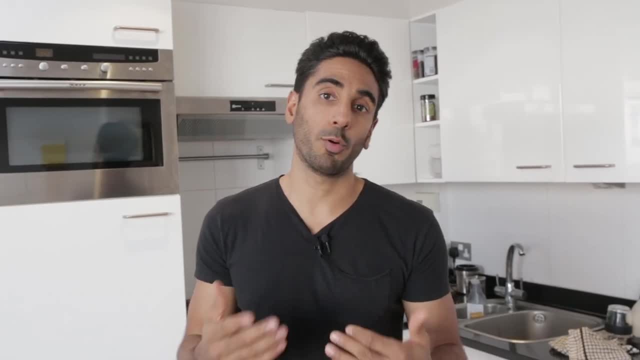 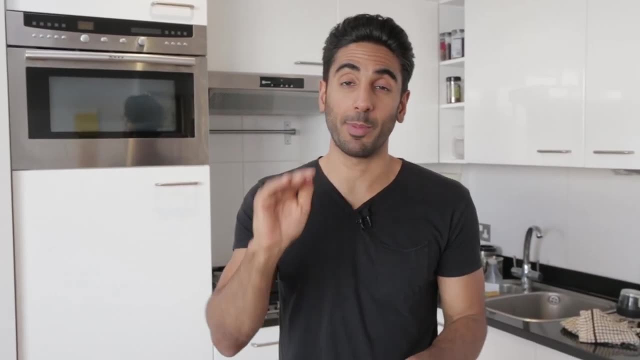 worthy. There are courses like mine that are more geared toward the general public, but not ones that I think are worthy for health practitioners. Which qualifications are therefore worthy? If you are serious about getting into nutrition, then there are two. There are Diplomas and 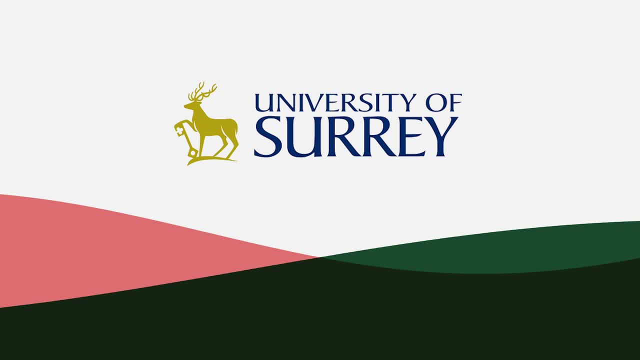 Masters. The Masters that I'm doing currently at the University of Surrey is perfect for those who still want to maintain their clinical career whilst doing a Master's part-time. Others, like the Masters at King's and UCL and others up and down the country, can get a Master's part-time, but I still think it's a good option. If you're a certified nutritionist, then you can get a Master's part-time. If you're a and the country are full-time, so you have to essentially go there four to five days a week. 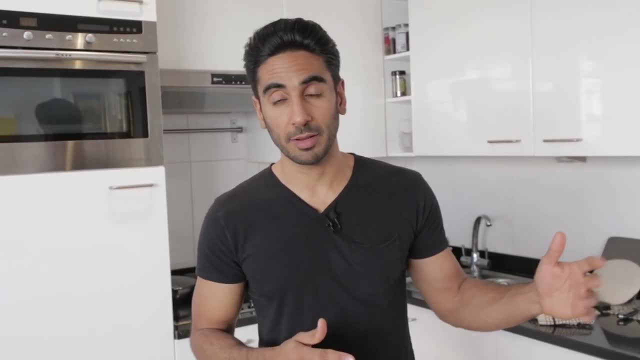 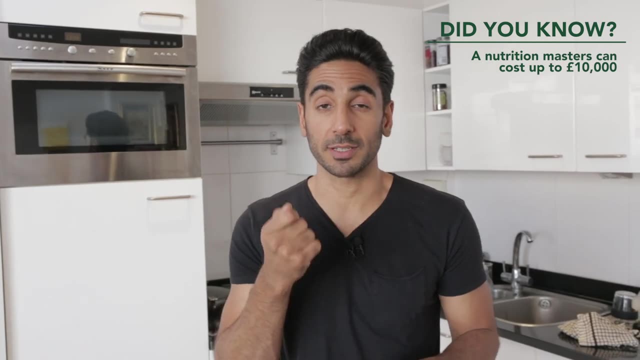 and for people who are actually practicing, unless you want to take a year out. if you can afford to do that, etc. it's not really practical. the masters that i'm currently doing at the university of surrey, the masters in nutritional medicine, is a lot easier for professionals to do because you 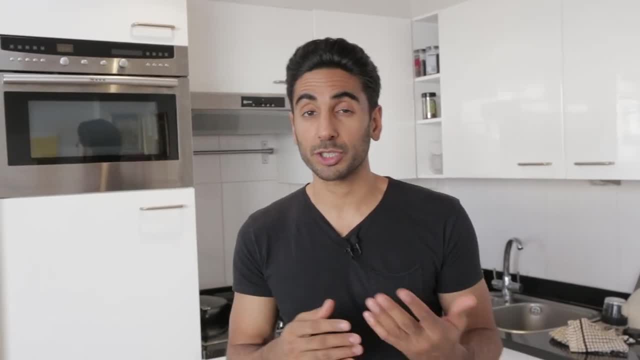 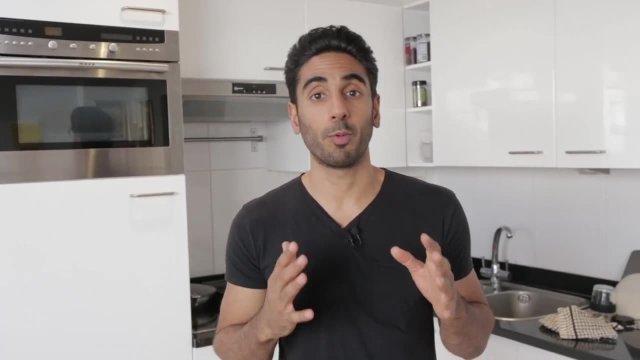 can do it in your own time. you go in for a week or so every six to eight weeks, depending on which module you want to do, and then you do essays in your own time as well. i think it's a lot more practical for those who are looking to combine their clinical career with extra education in 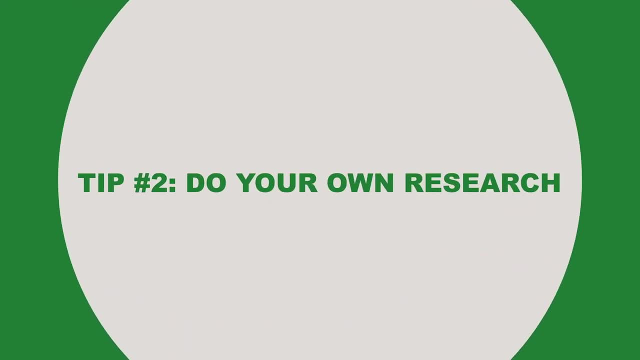 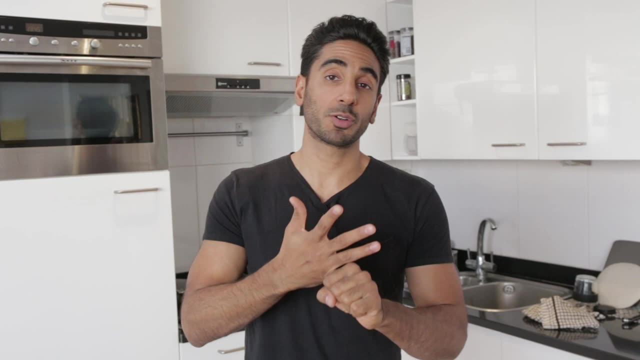 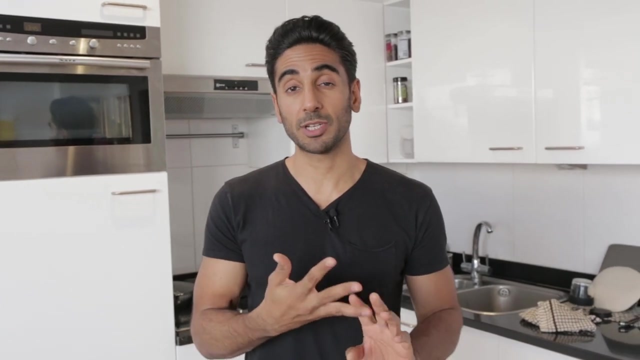 nutrition, but those are more formal. do your own research. okay, so i started by just sifting through all the journals and reading through different websites. okay, review articles are fantastic and you can find them on the bmj website if you look at pubmed bmj nutrition, which is a new 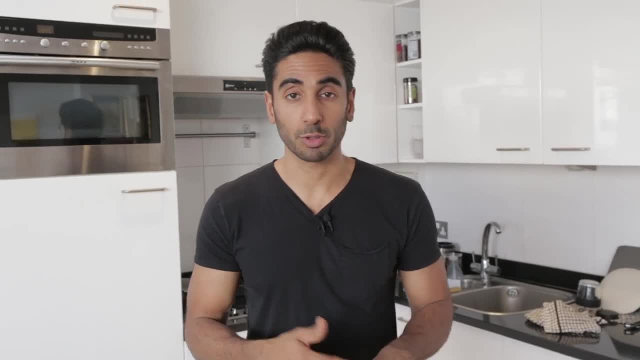 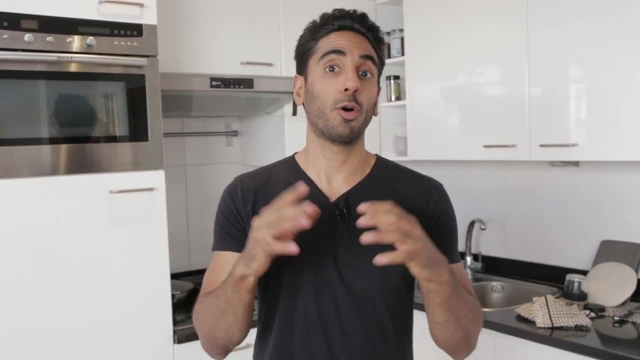 website and you can find them on the bmj website. if you look at pubmed, bmj nutrition, which is a new journal that came out in 2018, is a really good resource for all things nutrition related. the american journal of clinical nutrition is also great, and a whole bunch of others as well, with 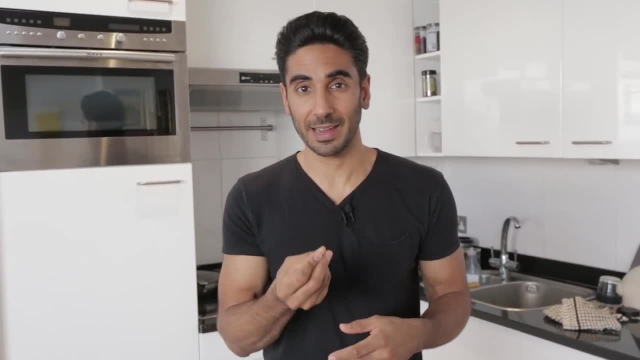 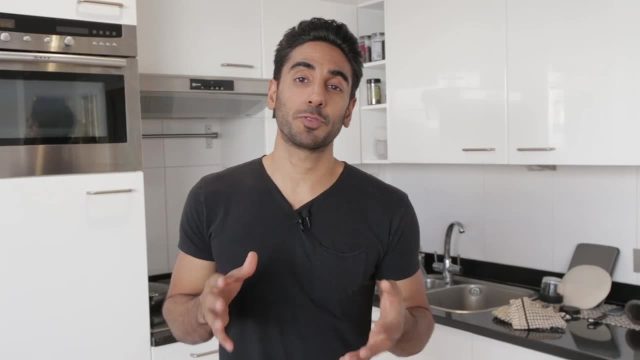 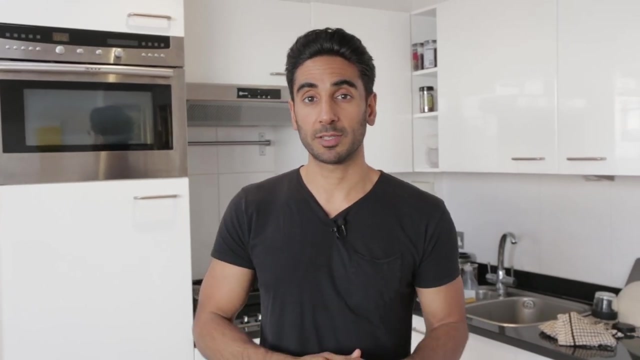 publications always take them with a pinch of salt, particularly when it comes to nutrition, because there is so much vague information out there. with nutrition research it is quite tough because we rely heavily on observational studies and a lot of lower quality evidence, which is why there is so much controversy with anything to do with nutrition overall, when 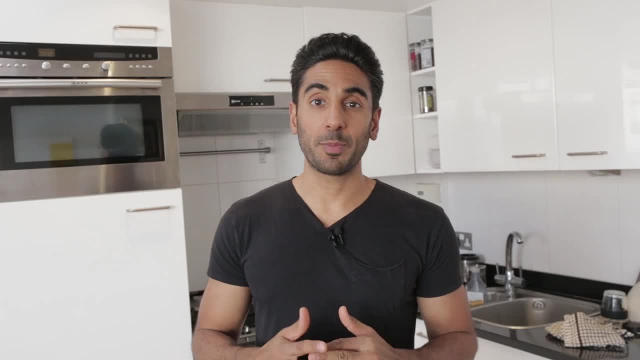 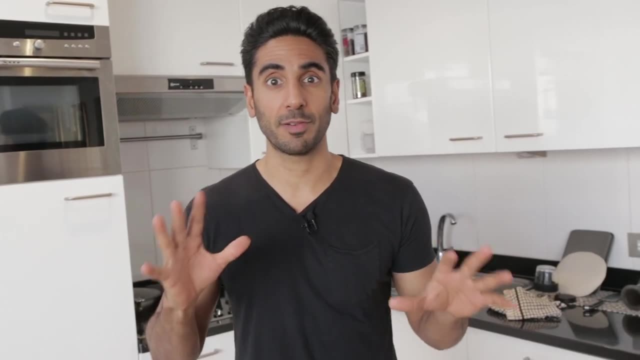 it comes to nutrition science, you need to be quite wary of people that brand themselves as nutrition experts or are quite dogmatic in their views. actually, nutrition is a very fluid and dynamic science, one where we need to be open-minded to a lot of situations. i never thought the keto diet. 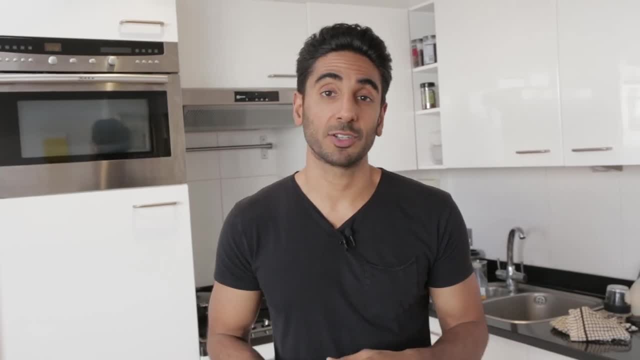 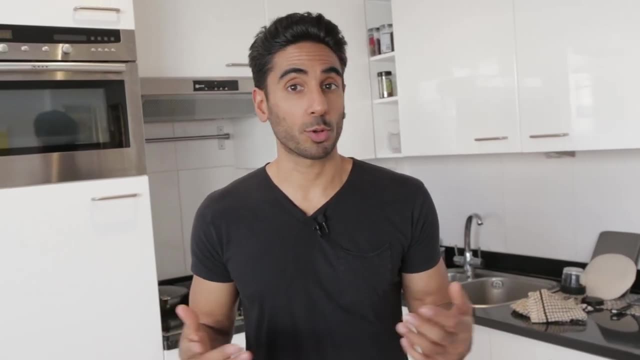 for example, was useful. however, there is some evidence to suggest that we can use it in certain therapeutic scenarios. so if you're interested in learning more about keto diet, for example, please be open-minded with everything and just make sure that you're being safe. there are simple core. 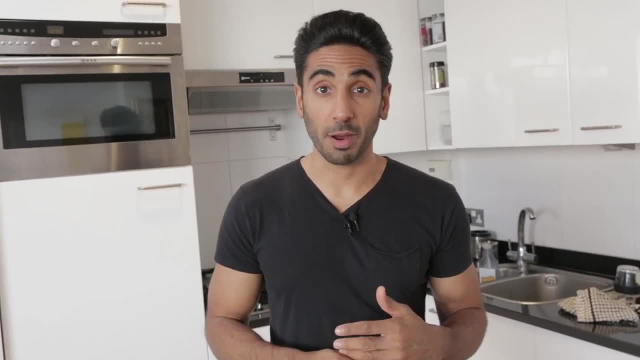 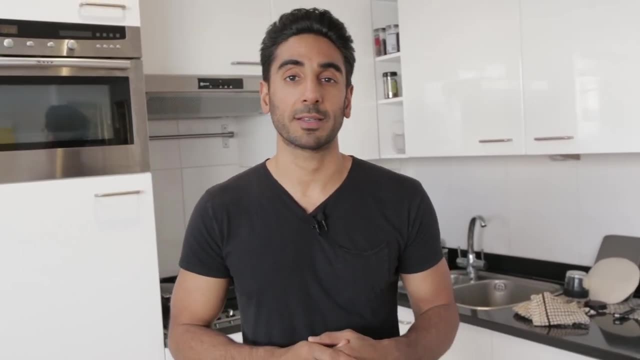 principles, things that i talk about in both of my books- that apply for the majority of people, and that's a very good starting point. however, there is nuance to the subject, as there is with anything in medicine. the third thing i recommend are all the incredible resources from registered 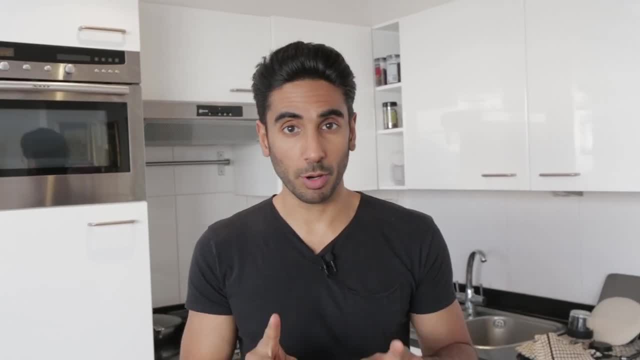 bodies that we have here in the uk and abroad. two of note are the bda website. they have food fact sheets that are directly available to the bda website. they have food fact sheets that are directly available to the bda website. they have food fact sheets that are directly available to the bda website. 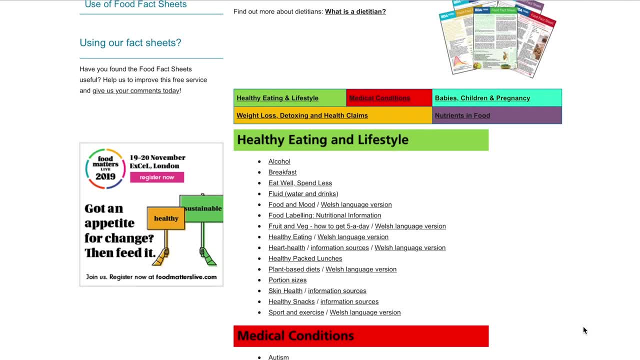 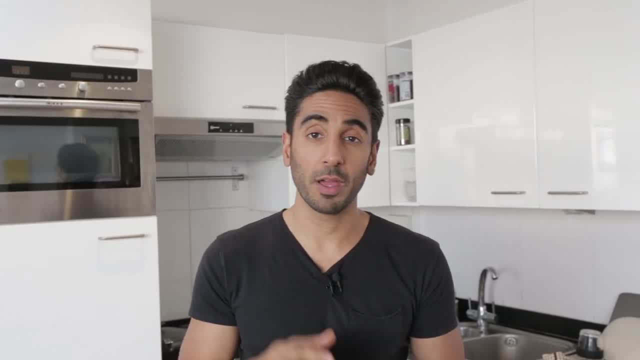 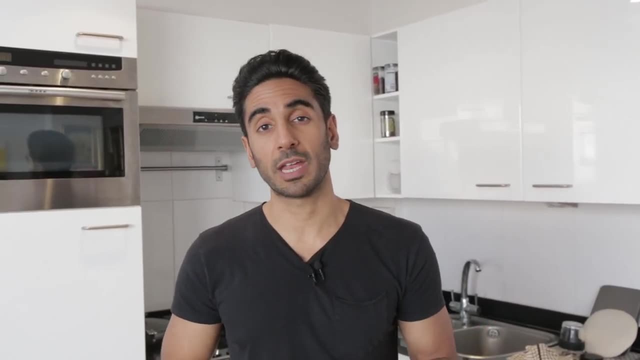 but they also have ones for professionals as well. they're really good for looking at things like dairy saturated fat, gluten-free diets, the evidence based behind low carb- really really good sources of information that are quite compact, easily readable and some resources that you can give to patients too. the other one is the nutrition society website. they again have got very basic. 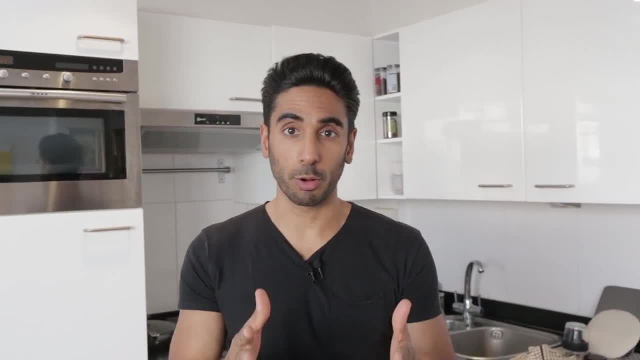 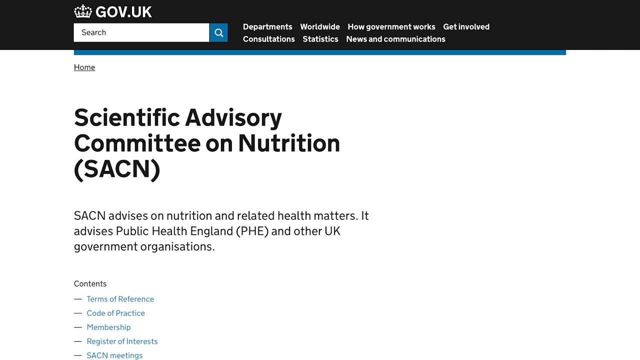 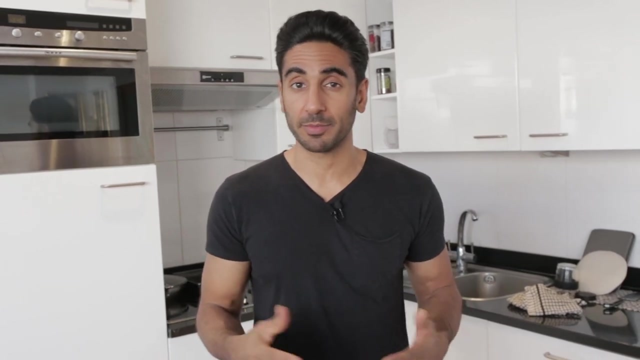 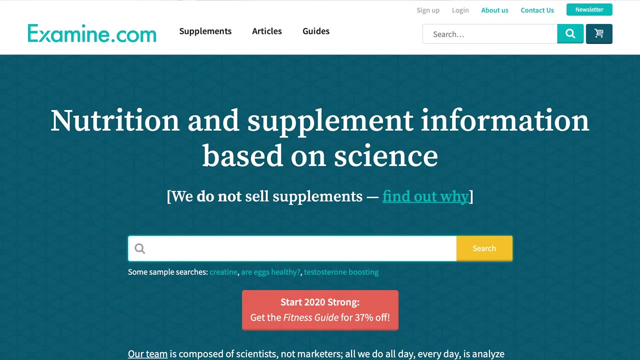 resources there for both professionals and for patients. go check those out. it's a good starting platform. another couple of resources within the same vein: second, that's s-a-c-n. that's a really good resource. they provide quite hefty reviews of things like saturated fat consumption in the uk and it's a uk focused body. and the other one i'm actually a big fan of is examinecom. 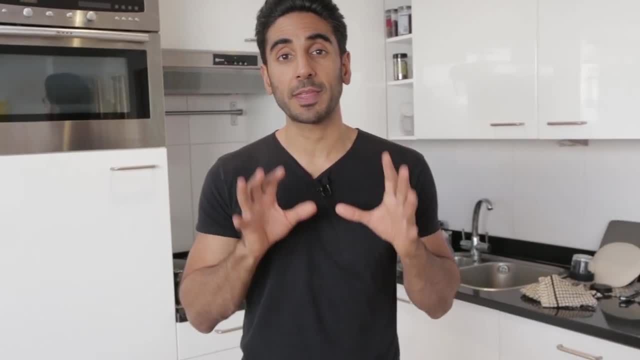 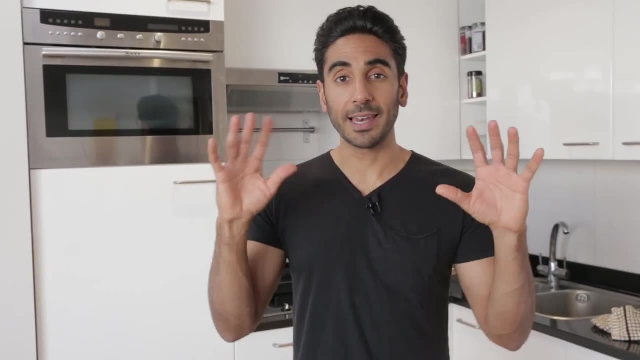 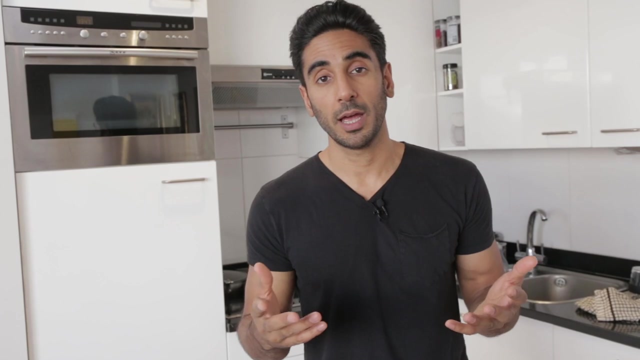 it's a really good website. it's geared more towards supplementation, but they do have articles on dietary advice as well. finally, if you really want to get a holistic view over a weekend or a week or so, go to a conference, the american journal of clinical nutrition. they held a conference in, i think it was florida at the time. this is going about five or. 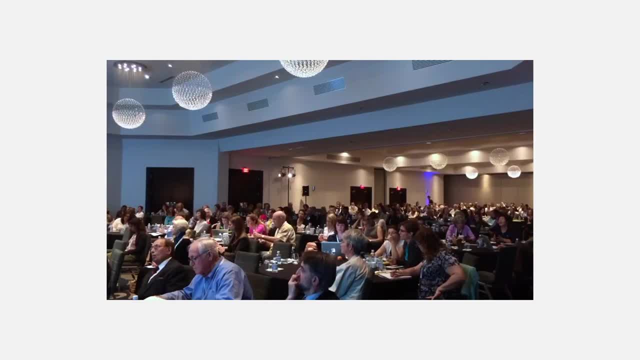 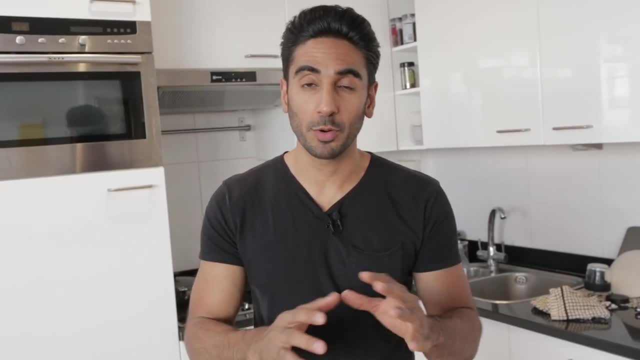 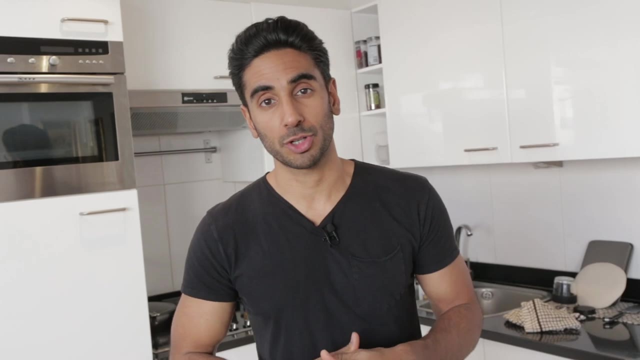 six years and honestly, that was an incredible immersive experience into what nutrition has to offer, as well as a networking opportunity by speaking to other people. i hope that's been useful. it gives you an overview of the journey that i've been on, but also a strategic way of tackling the issue of poor nutrition. training amongst health professionals. 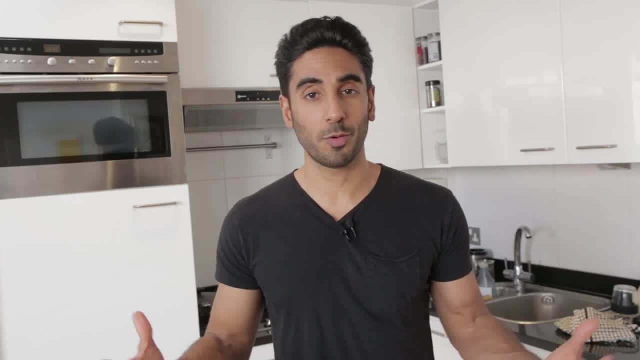 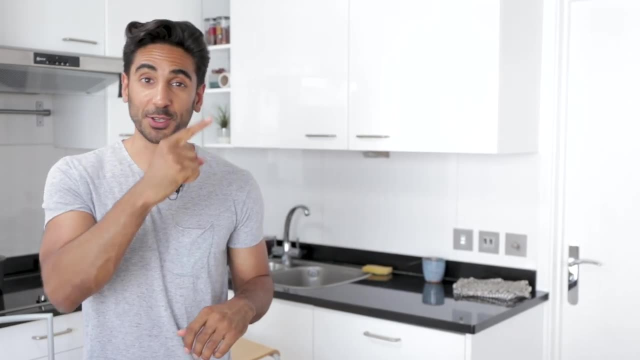 go educate yourself, have fun, learn about the wonderful world of nutrition and be open-minded as possible. thank you so much for watching this video. there's so many others for you to enjoy right here. check out thedoctorskitchencom. sign up to the newsletter, where i